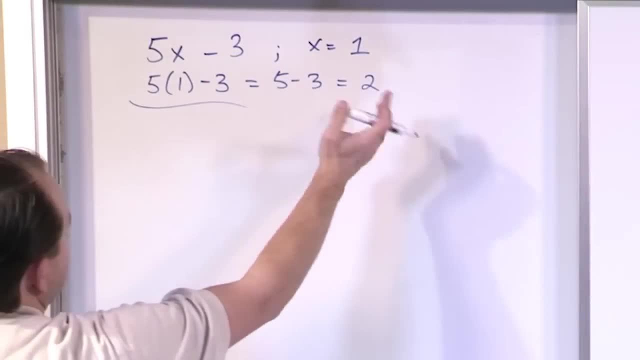 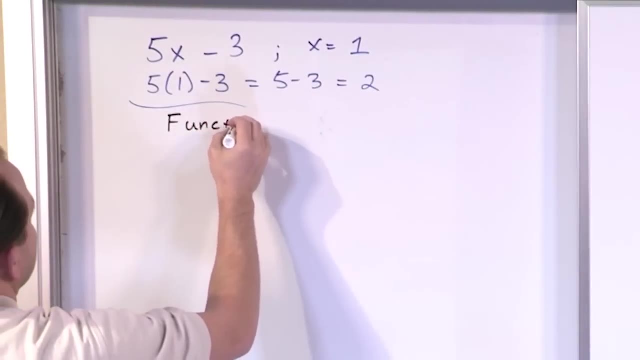 So this is just an expression, a polynomial right, And we just set the value equal to one, we calculate it. But let's go ahead and define something called a function. You know, in everyday language, what is a function right? What is a function? Well, 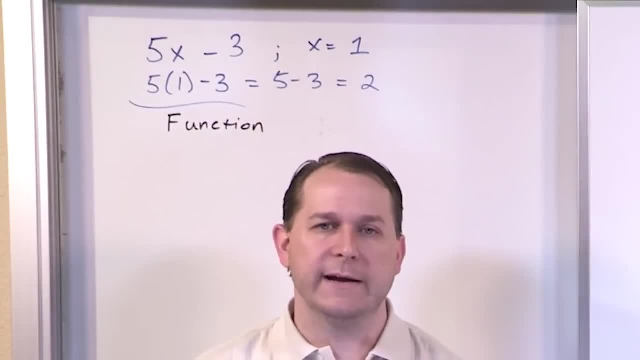 a function is something that describes how something works right, Like my pencil sharpener has a function. The function is I stick a pencil in and it sharpens the pencil right. My car has a function. The function of my car is to propel me and get me around town. Everything has a 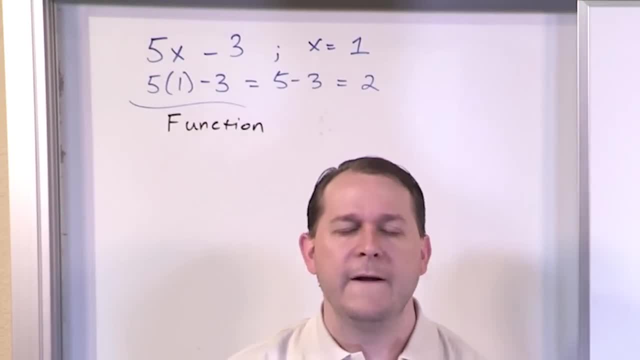 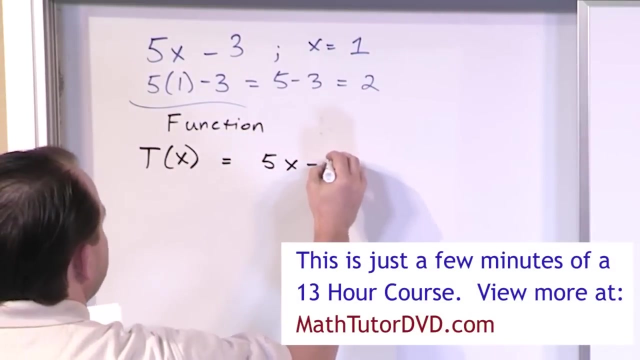 function, It does a job. When something has a function, it does a job. So functions in algebra do a job. They calculate things. And let me give you an example of that. What if I have a function t of x- and I'll explain what all this means in a minute- is equal to 5x minus 3.. 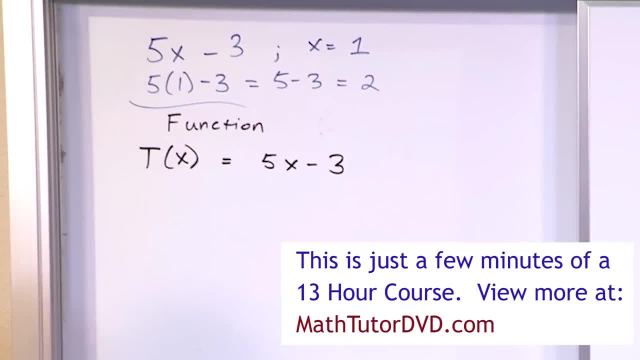 Notice, I used the same exact thing: 5x minus 3.. I used the same thing that I used up there, because I'm trying to basically tell you: it's the same thing that we've been doing all along. It's just written down a little bit differently. 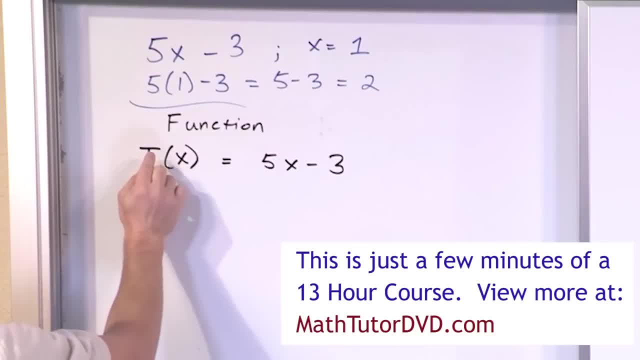 This represents, on the left-hand side, a function. When you see a variable, parentheses and then another variable, you might think this is just t times x, because parentheses mean multiplication in algebra- And they do. But this is a little bit different. This is not really. 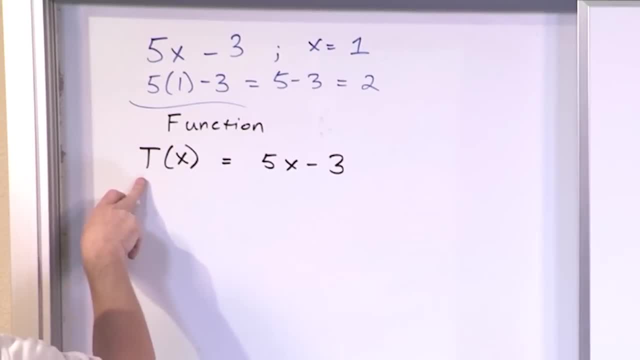 saying multiplication of t times x. This is saying that t, whatever it is, is a function of x, right? Let me ask you a question. Do you think, in this room that I'm standing, that the temperature of every point in this room is the same? right, If I take a digital thermometer? 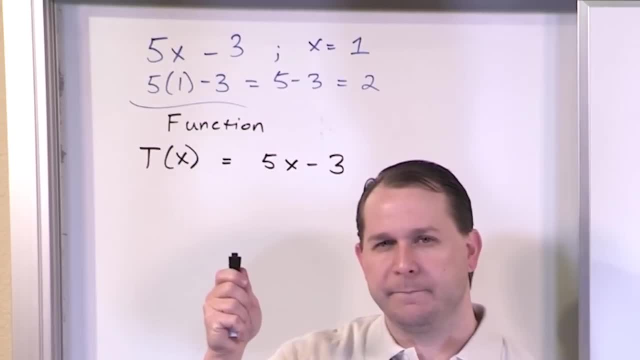 that's extremely accurate and I hold the thermometer here. it might read, I don't know, 75 degrees Fahrenheit or whatever, 28 degrees Celsius or something, And then I might move it over here and it's going to read a slightly different temperature. It's going to be close. 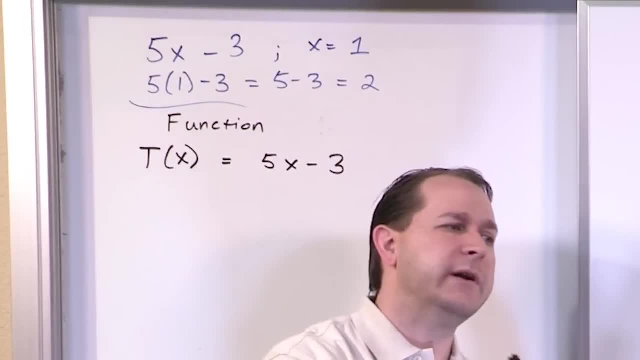 because we're in the same room, but it's going to be different, okay. Well, it might read 73 degrees over here. If I move it up, it might read slightly different temperature, and if I move it over this way, it's gonna read a slightly different temperature. so, and wherever I, 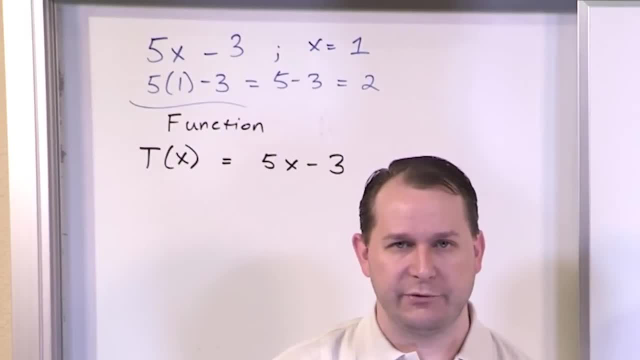 move my temperature probe, I'm going to read a different temperature. so the temperature reading is a function of position. it's a function of wherever I put the probe. when I measure the temperature here, it's gonna be different than when I measure it over here. it's gonna be different when I measure it. 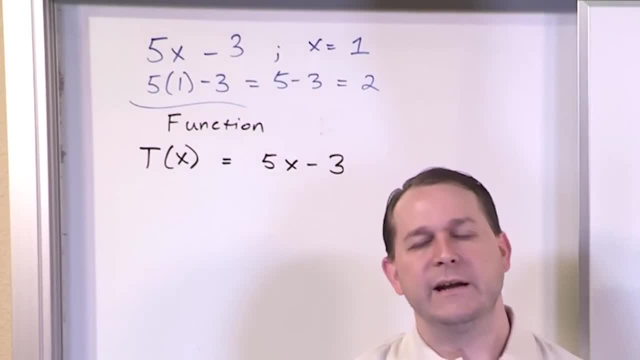 over here. so it's a function of position. in algebra and in physics and other classes we usually use X to talk about the position. so basically you would say the temperature is a function of X. you know, X might be 0 right here and right, and then 1 centimeter over here might be X is equal to 1, 1 more centimeter X is. 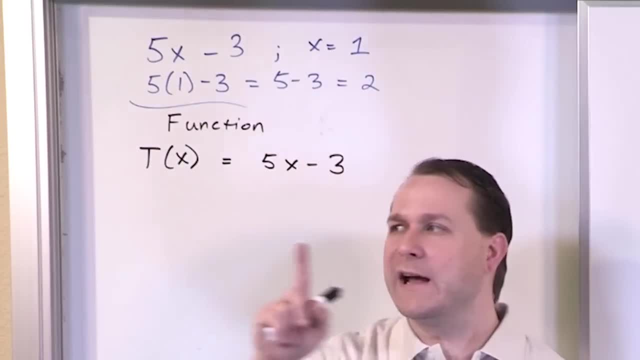 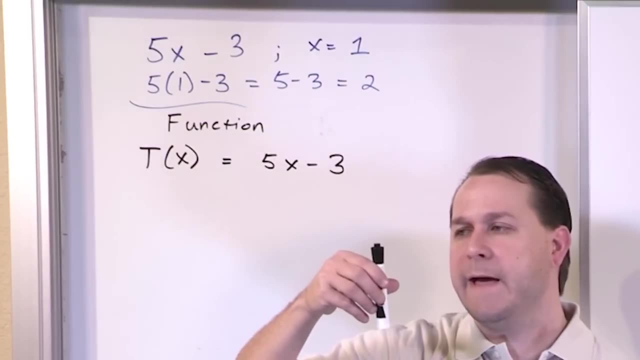 equal to 2, X is equal to 3, X is equal to 4, X is equal to 5. so you kind of have like a number line right in front of you here. where X is equal to 0 is over here 1, 2, 3, 4, 5, and then, if you go the other way, X is equal to negative 1, negative 2. 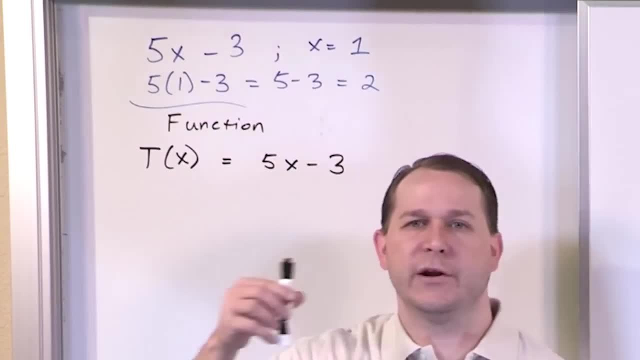 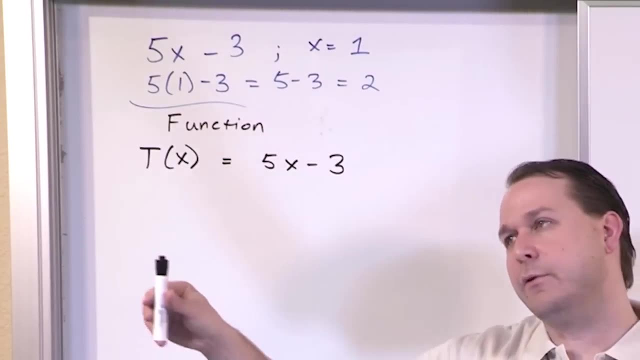 negative 3, negative 4, negative 5. so you have kind of like a grid right in front of you: values of X and as you move the probe this way it's bigger X. when you move the probe that way it gets to 0 and then it goes. 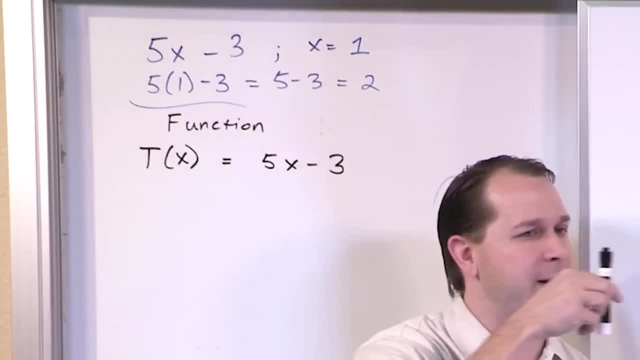 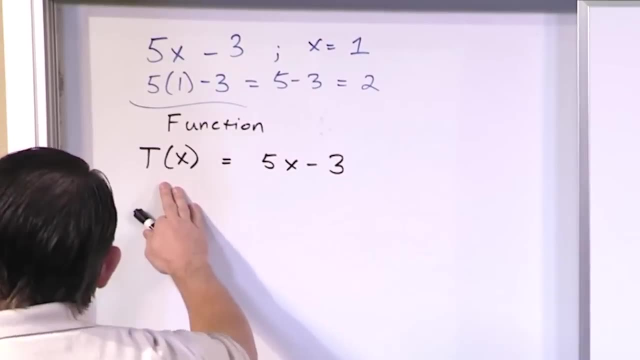 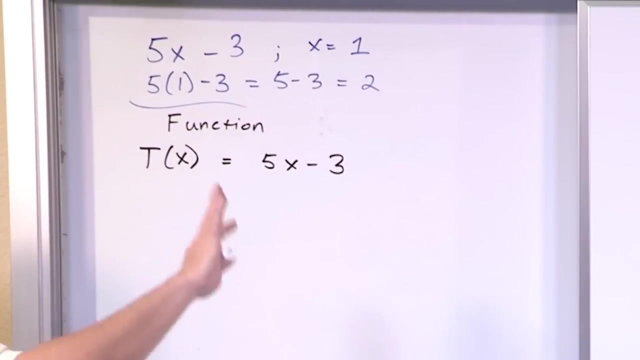 negative, X, right, and so wherever I put my probe, I'm getting different temperature readings. it's a function of X, a function of position, and that's what I've written down here without telling you this. T is representing the, let's just say, the temperature in this room along the line, right, oh, not everywhere. 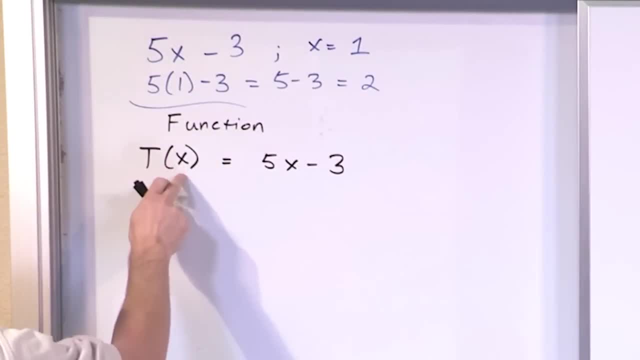 just along some line, and it's a function of X, it's a function of wherever I put the probe. So if I measure the temperature here and I measure the temperature over here, and then over here and then over here, it's all going to be the same. 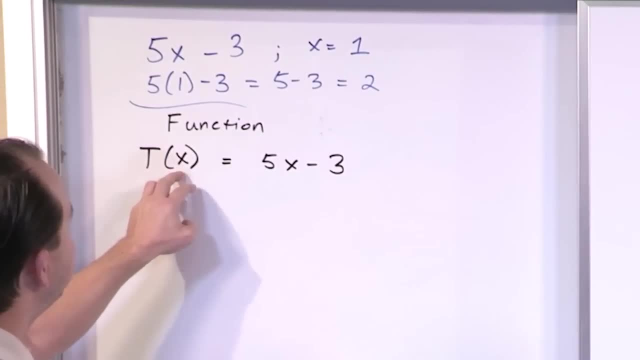 Now I'm just saying, for the sake of argument, that this temperature, as a function of x, is equal to this expression. So what I can do is this is telling me what it's a function of. This variable is always going, whatever it is. 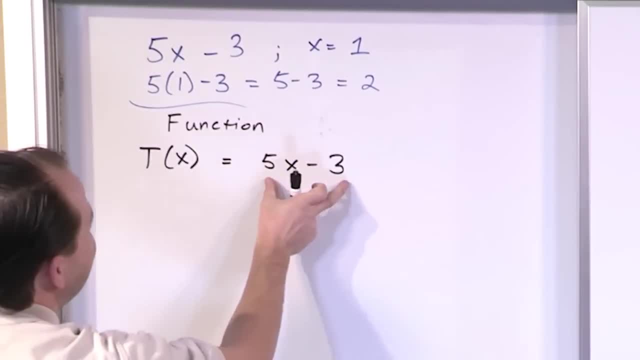 is always going to pop up over here because I'm saying it's a function of x, So it has to be present over here in the math. So if I put in x is equal to 0 here, what am I going to get? 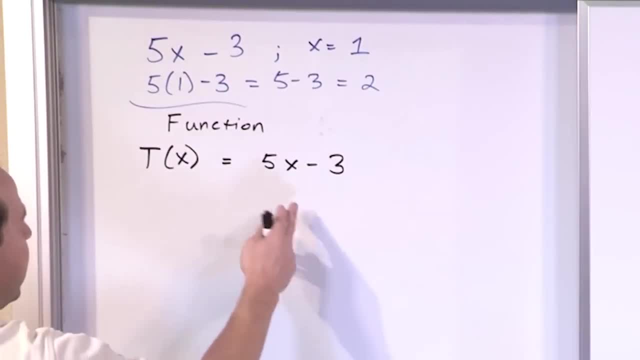 5 times 0 is 0, minus 3 is negative 3. So obviously this does not really represent the temperature in this room, But if it did, then what it's saying is that if x is equal to 0, the temperature 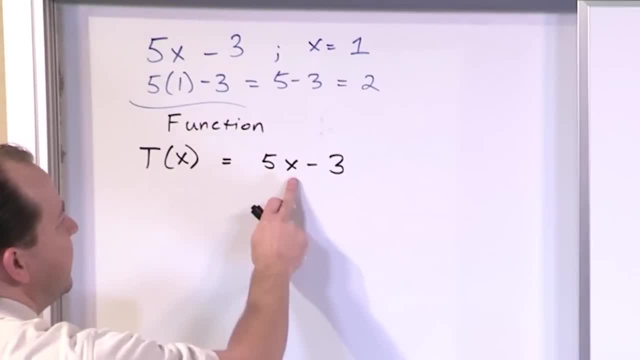 is negative 3 degrees. That's what it's saying. If I put x is equal to 1 in here, 5 times 1 is 5, minus 3 is 2.. That means that if x is equal to 1,, 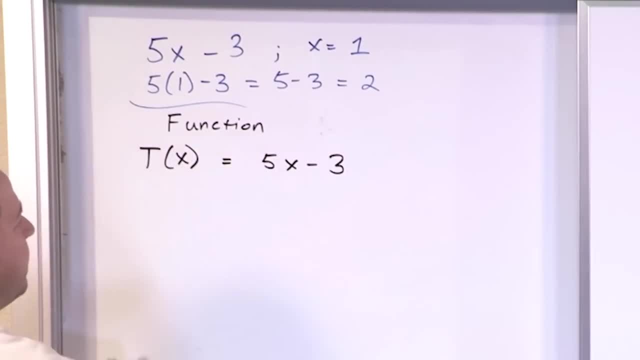 when I go to 1 centimeter to the right, the temperature is going to be 2 degrees, And so I can plug in different values of x and put them in here and calculate different values of temperature, because that's what I've actually. 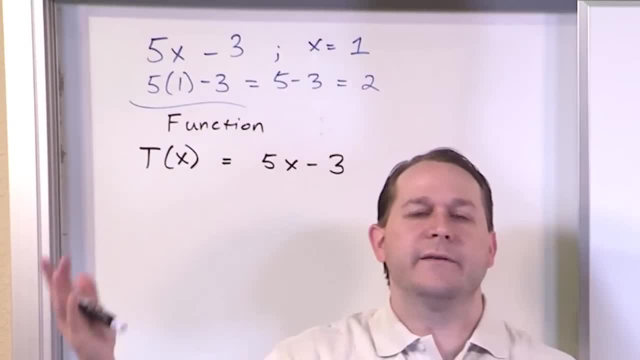 defined this function to represent. So, in the biggest possible picture, functions in algebra are very, very practical, because that's what you really use algebra for. All the stuff we've done so far it's kind of been just sort of like just to teach you. 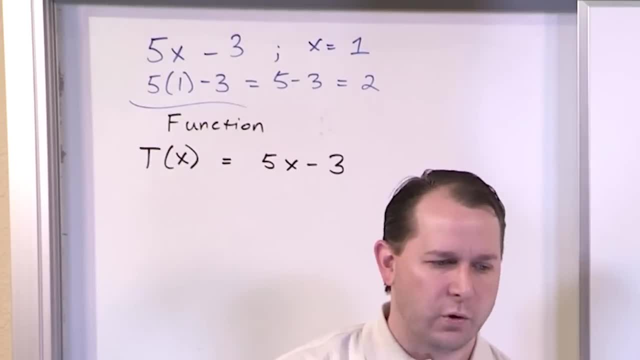 how to use algebra. But really, functions are really when you start rolling up your sleeves and using algebra. Here we're talking about temperature as a function of position in the room, But I might have a function, That's pressure as a function of altitude. 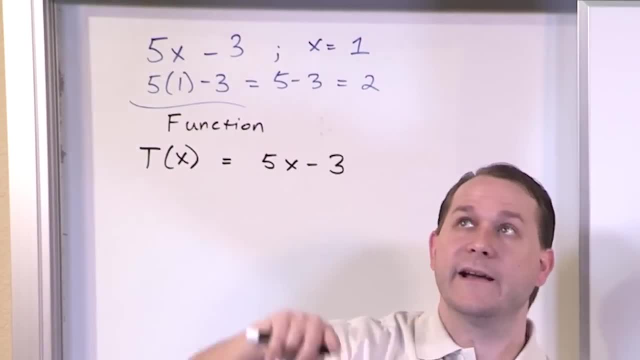 When I go up towards space, the pressure gets lower, lower, lower as I go, And then eventually I get where there's no air and there's no pressure at all. Well, I can make a function so that I can plug in values of my altitude. 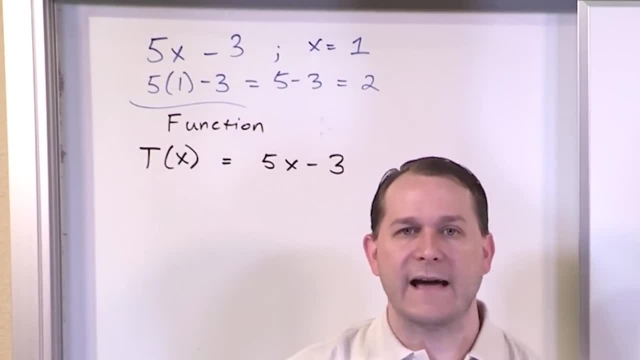 and then I will calculate the pressure. That is a function. It's a function of altitude. I could have a function of velocity, calculating something as a function of velocity. I could have a function of anything I can make up that is represented in the real world. 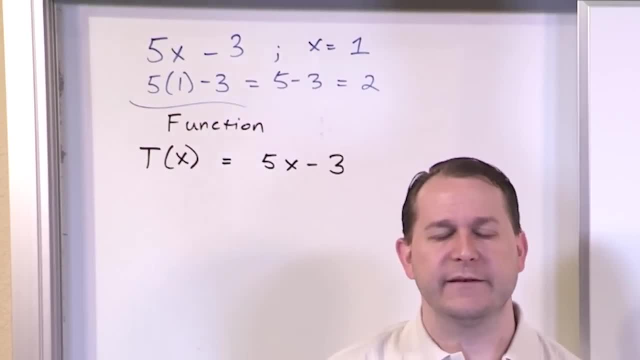 I can calculate things that are basically dependent on other things. They're a function of other things. So I did a lot of talking, but I finally want to do some actual math, to kind of show you how to nail it down If you want to calculate this temperature getting back. 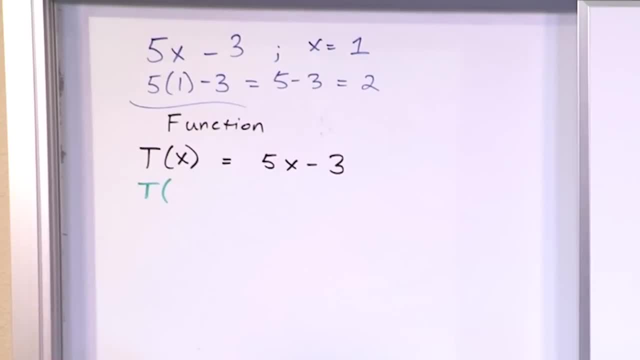 to our temperature, example, as a function of position, then if I want to calculate it at x is equal to 2, then I just put a parentheses in here. This is not t times 2.. This means the temperature is a function of position, at x is. 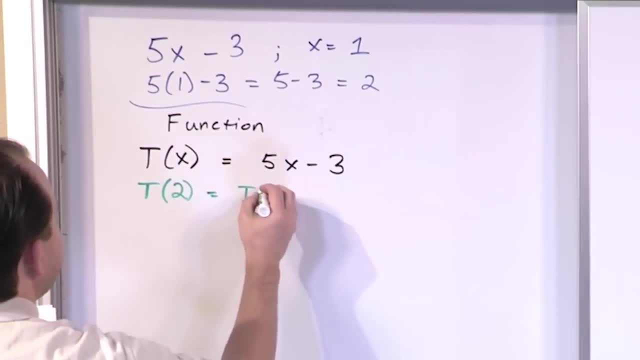 equal to 2.. That's the same thing as saying that x is equal to 2.. It's the same thing as saying x is equal to 2. in here You just write the 2.. I'm just kind of showing you here. 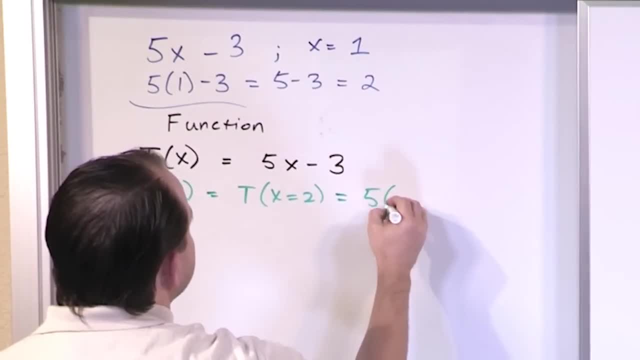 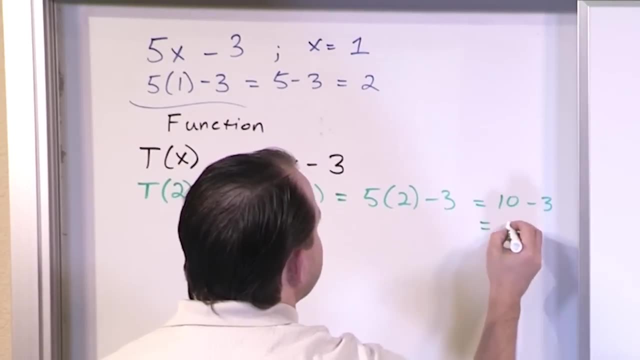 Then what you do is 5 times 2 minus 3, 10 minus 3.. And so what you're going to get is 7 over here. So if this were really a function of temperature, then x is equal to 2, wherever I've defined that to be. 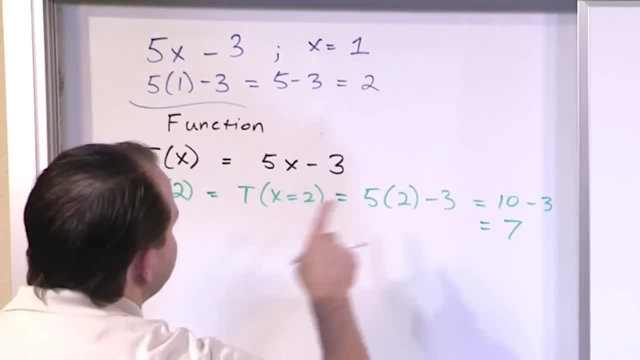 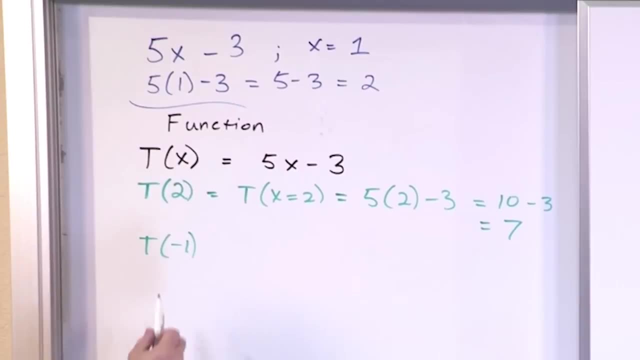 the temperature is 7 degrees. What if you had? x is equal to 2 minus 3?? What if I had a position of negative 1?? That's not too magical. It just means, if this is my 0 point, that I've defined. 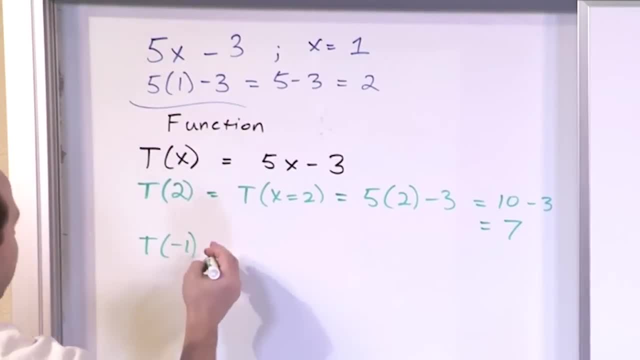 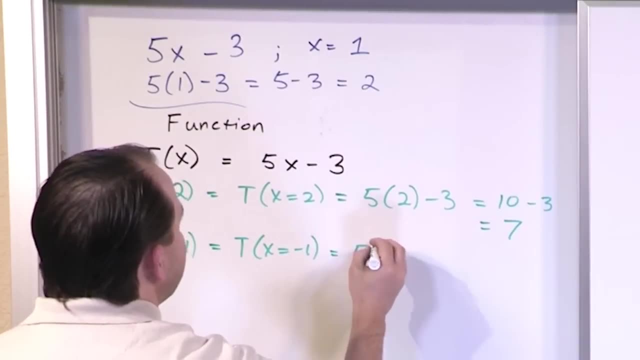 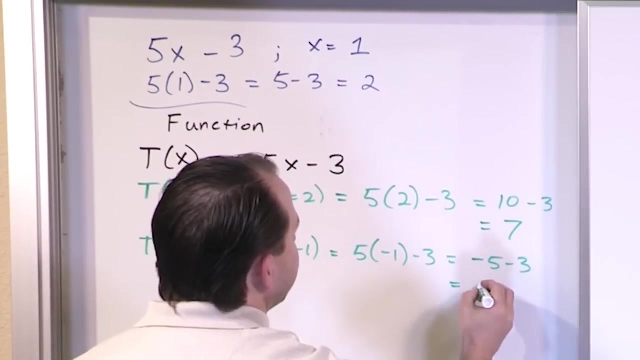 then negative 1 is this way, instead of this way going positive, So it's just going the other direction. So I'll say x is equal to negative 1.. 5 times negative: 1 minus 3.. This is negative 5 minus 3.. 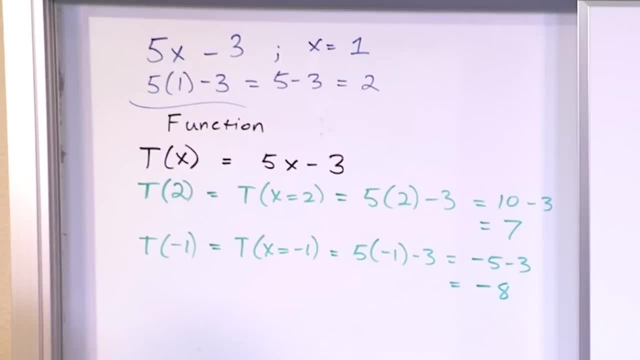 Negative 5 minus 3 is negative 8.. Right, So it's interesting, I'm finding out right here. let me go ahead and circle this, just so you can kind of keep track of it easily on the board. Basically, what we're saying is that x is equal to positive 2.. 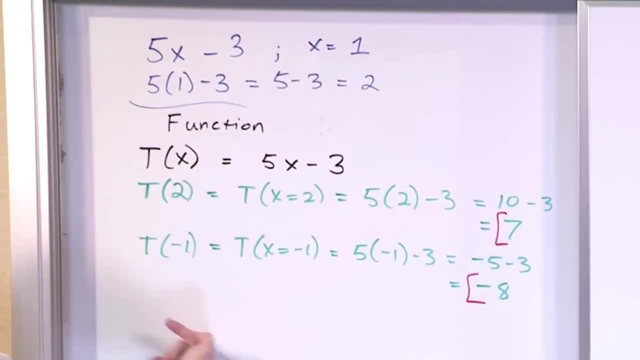 The temperature is a positive number, positive 7.. And when I go the other way, the temperature, at this way, a little bit farther left, at negative 1, and x is equal to negative 1,. it happens to be a negative number. 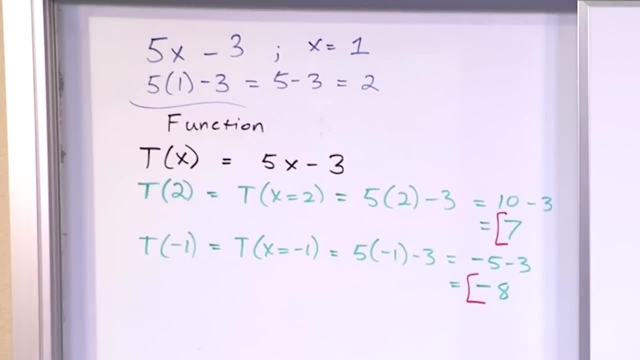 So you can see. no matter what value I put in for x, I'm always going to calculate some temperature, And this we're just pretending actually represents the temperature in the room In real life. if you were doing an experiment, you'd have to measure everything. 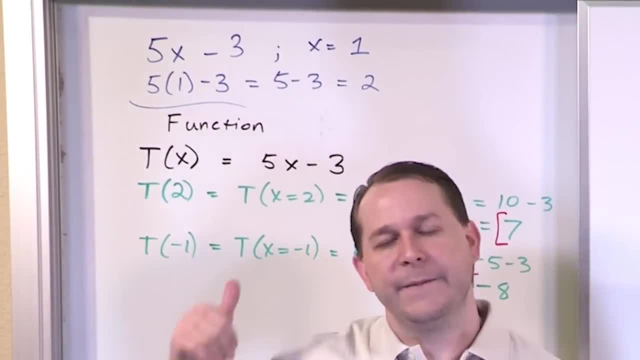 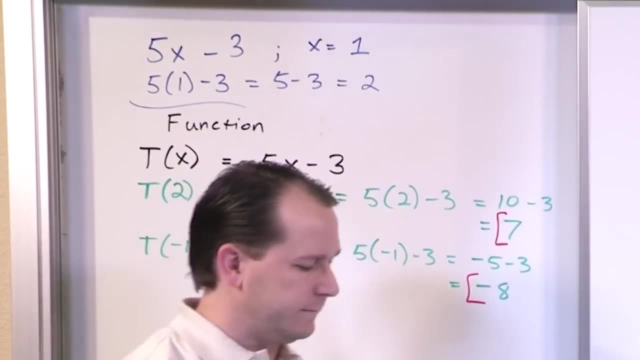 And you calculate a function that describes reality. This obviously doesn't describe reality. It's not 7 degrees here and negative 8 degrees over there, But it's illustrating the point for you. The main thing for you to understand is: these represent calculations. 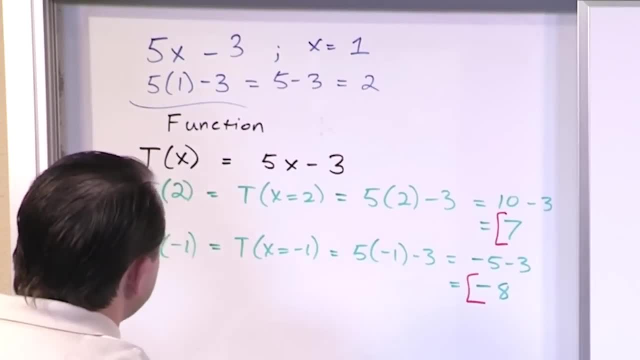 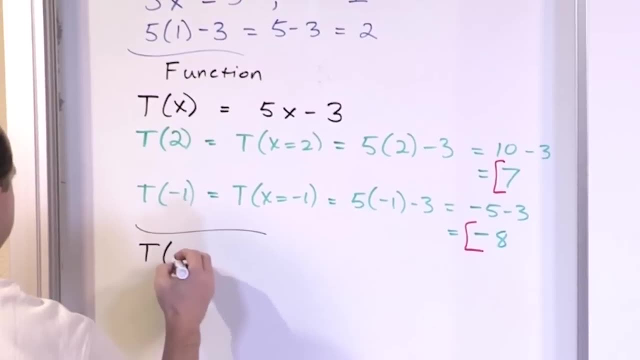 You put in a value of x, You get a value back. That is the general idea of a function, And you don't even have to put numbers in here. You can put anything you want here. I can say t, I can put a variable in there. 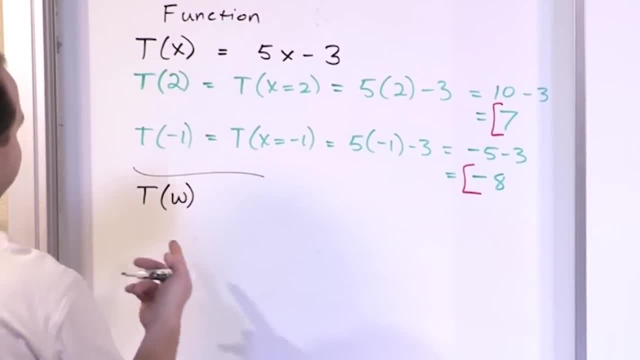 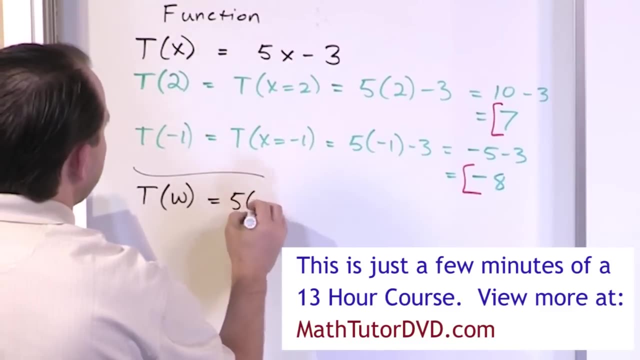 And I'll call it w. It doesn't matter If your teacher says, hey, evaluate this function t at w, then you're just going to take whatever's in here and stick it in here 5 times w minus 3..